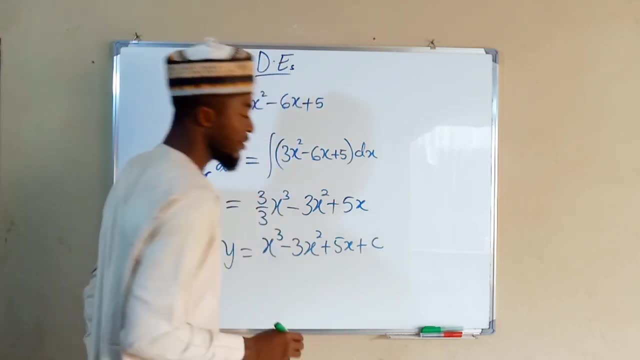 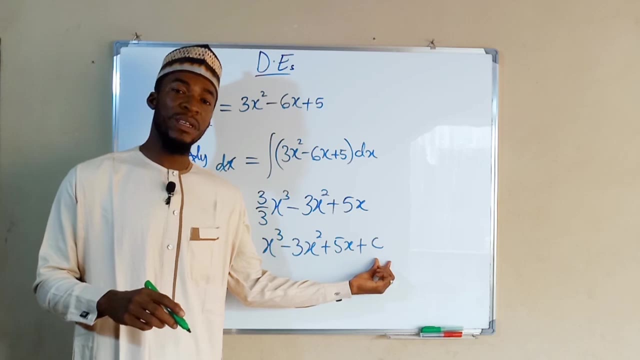 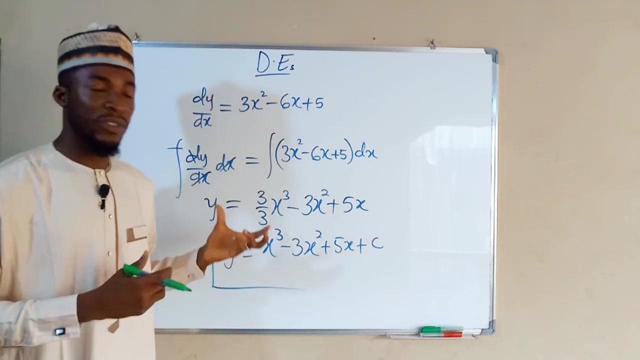 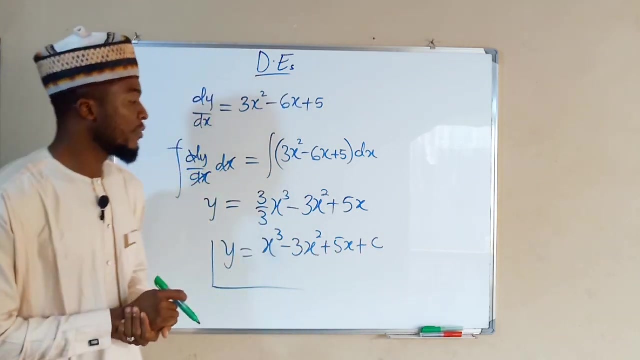 so we have therefore 5, X plus our constant of integration, C. so we call this a general solution because the value of C is unknown. So at first we are given some additional information about this differential equation. we can use this information to find the value of C. then we substitute: 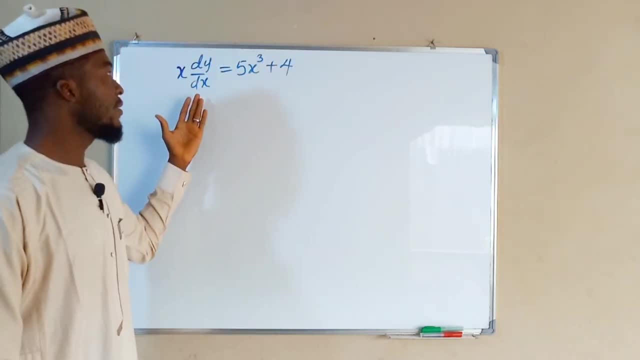 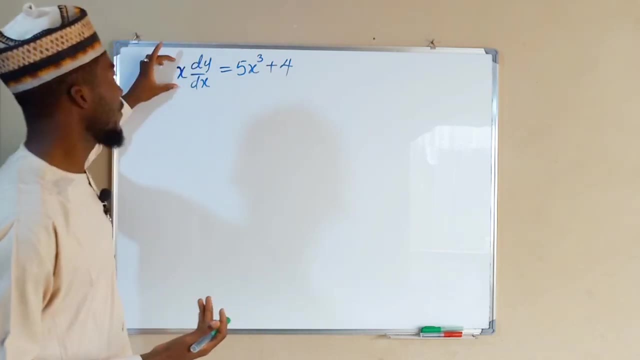 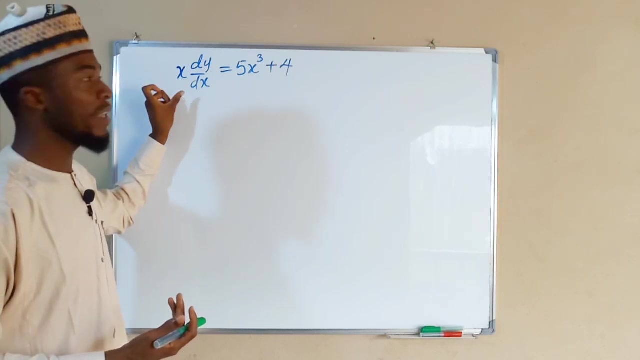 it back to obtain a particular solution. see, our second question is not in the form of dy over dx, equal to our f of x, because we have another x here multiplying our derivative. so all we have to do is to divide both sides by this x in order to eliminate it here. so by dividing both sides by x, we have from the left hand side, dy. 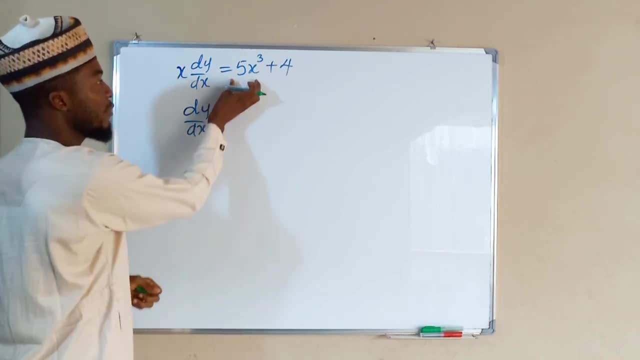 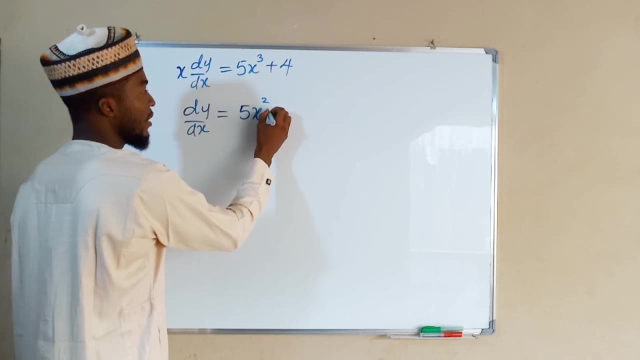 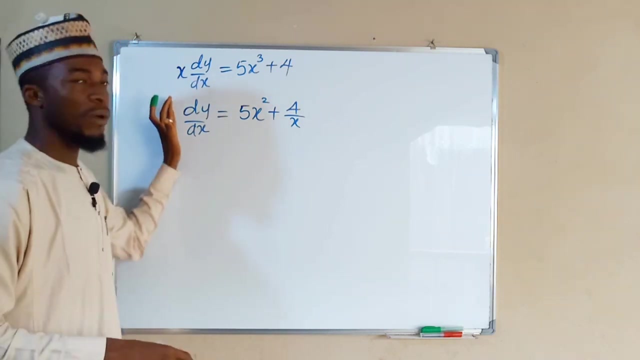 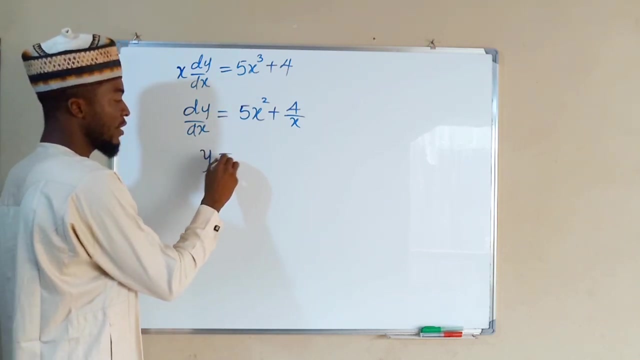 over dx equals to. if you divide this term by x, the power of x will reduce by one. so we have five x to the power of two, and the last term is going to be four over x. now we are free to apply our integration to the both sides. if you integrate this side, you are going to obtain y, and to the. 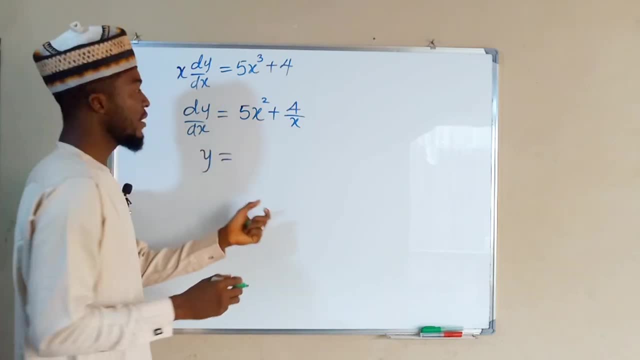 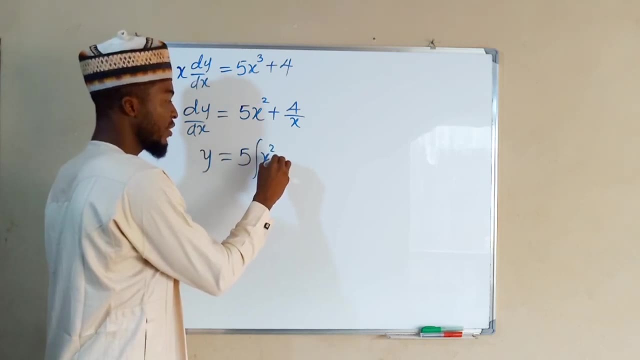 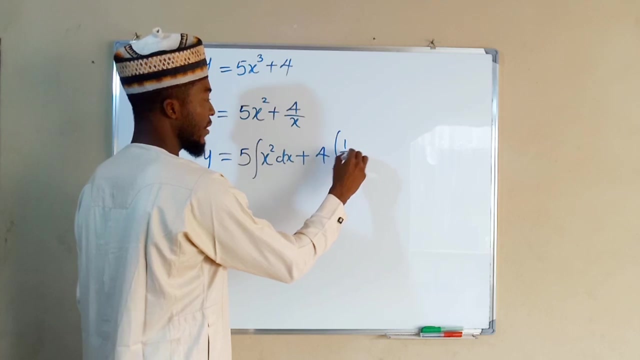 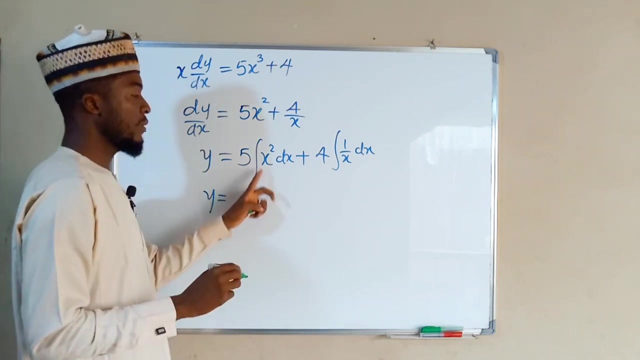 other side, we can integrate these terms independently. so let us integrate the first term by factoring five out, then we integrate x squared with respect to x plus. we can do the same here. we factor 4 out, then we integrate 1 over x with respect to x. y equals 2.. If you 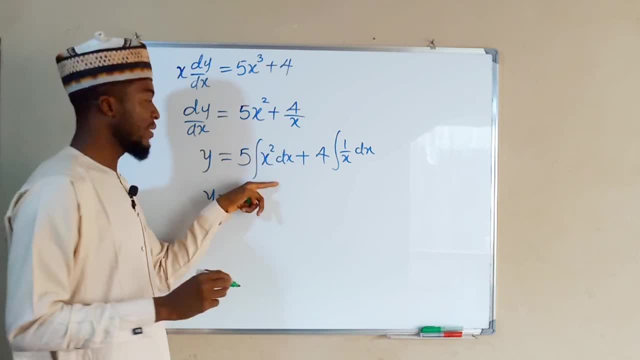 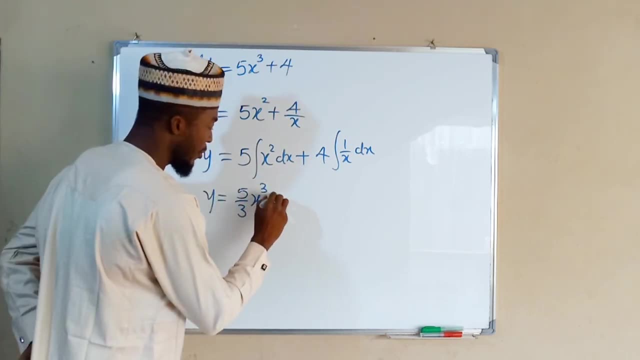 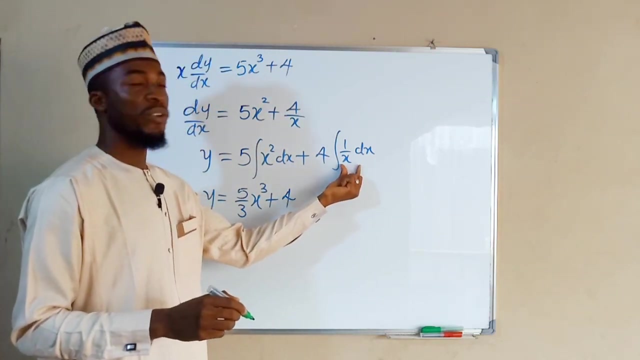 integrate this, you're going to obtain x to the power of 3 divided by 3, which is the same thing as 5 over 3, x to the power of 3, then plus here we have 4 times the integral of 1 over x, which is just the natural log of x. So we have the. 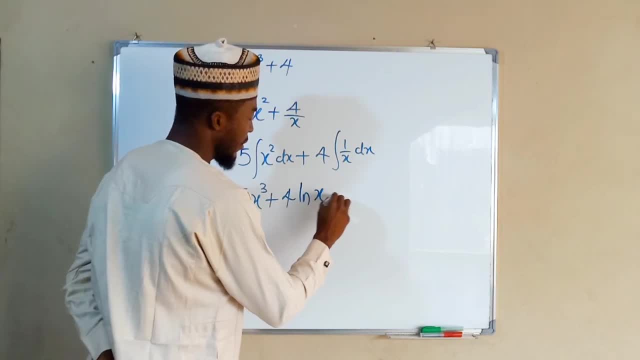 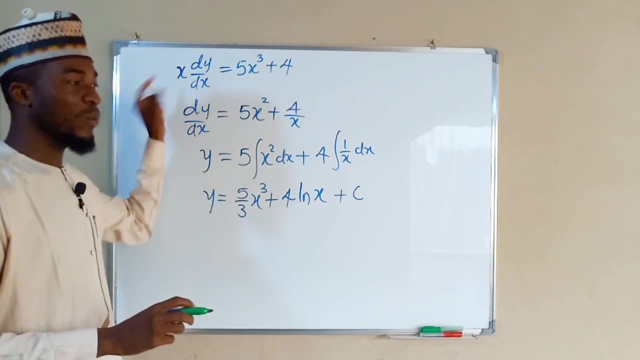 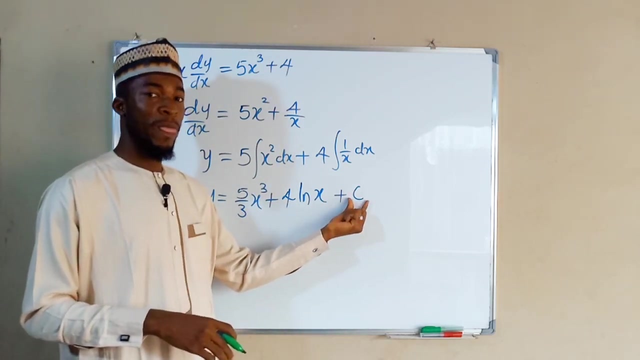 natural log of x, then plus our constant of integration, c. So this is the general solution for this differential equation. The same thing if other conditions are given. we use those conditions to find the value of c, then substitute the value of c back to obtain a particular solution. 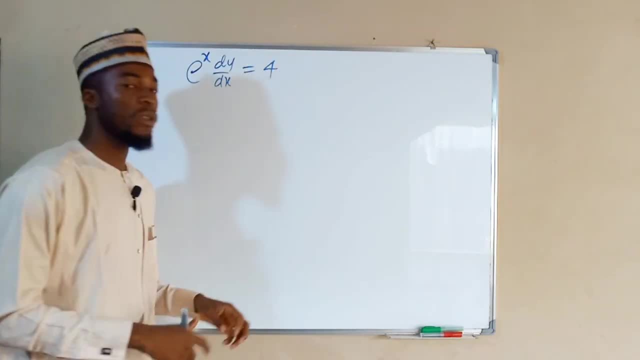 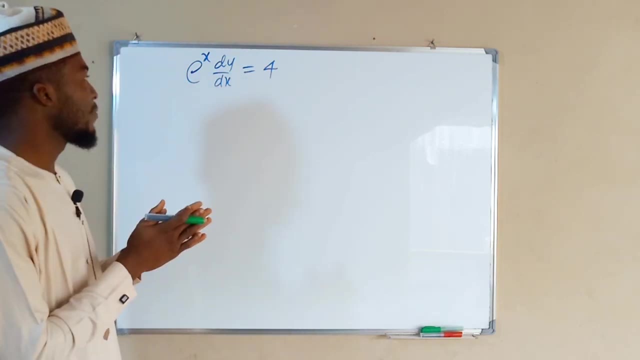 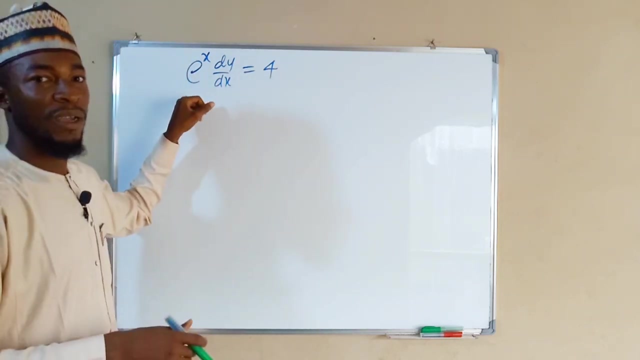 So now let us look on to the last problem. The last problem as well, is not in the form of dy over dx equals to f of x, because we have a real exponent multiplying our derivative. All we have to do is to divide both sides by our real. 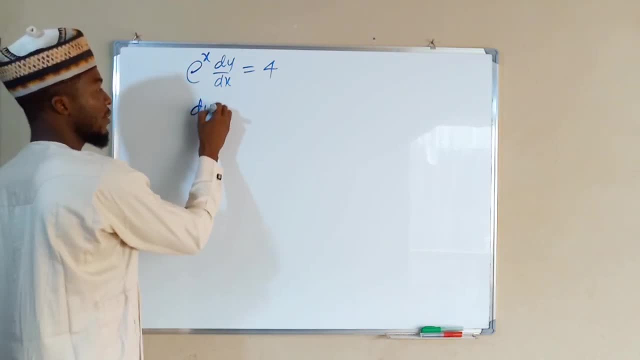 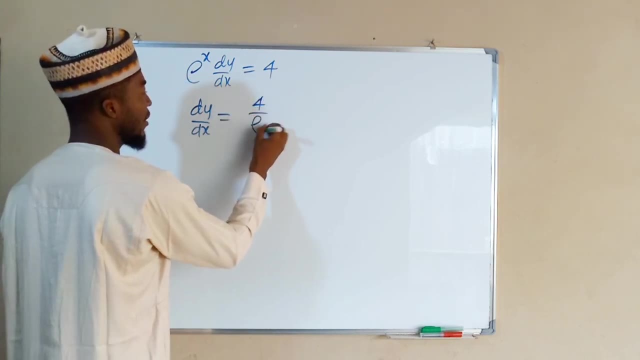 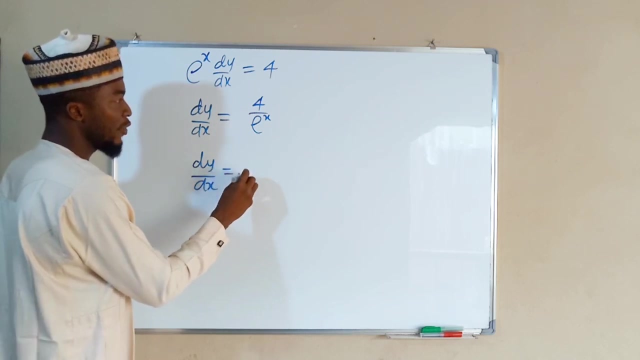 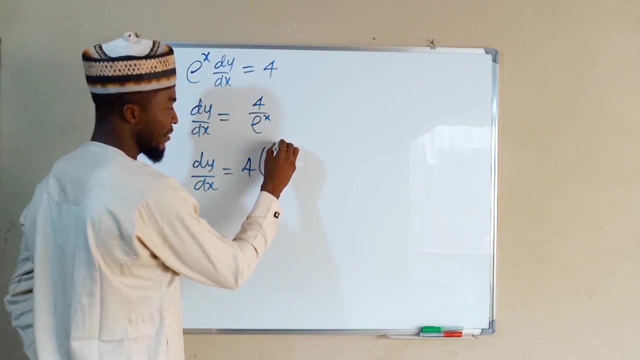 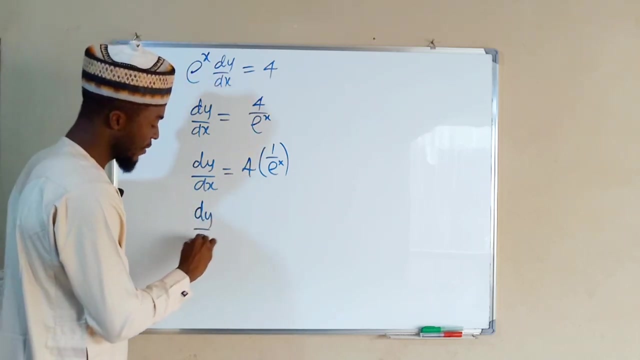 exponent. So we have, from the left hand side, dy over dx and this is equal to 4 over exponential x. dy over dx will now be equal to 4 times 1 over exponential x. I have just factored 4 out. dy over dx will now be equal to 4.. Law of indices: this can be. 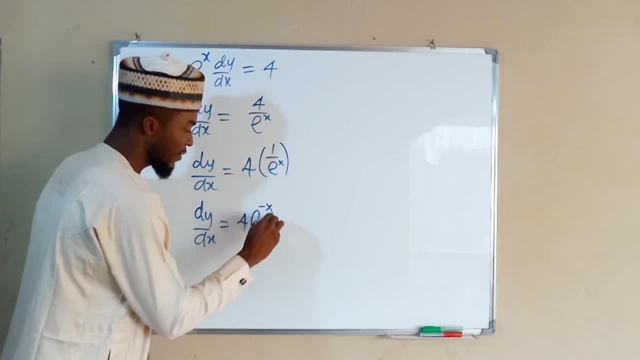 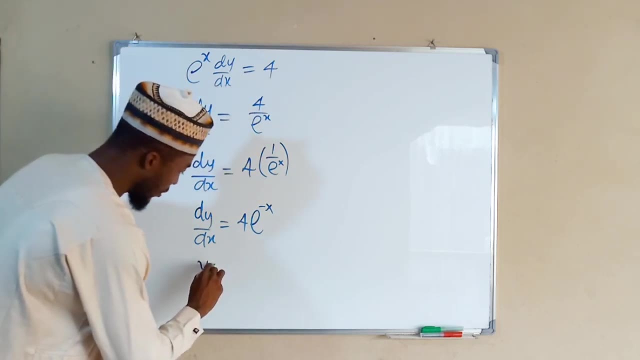 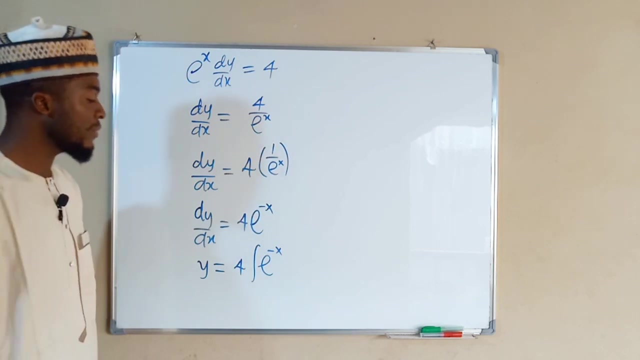 written as exponential negative x. So what is left for us is to integrate both sides. So from the left hand side we have only y and to the right hand side we have 4.. Then the integral of exponential negative x, This is y- equals 4 times if you take the integral of exponential of a function in 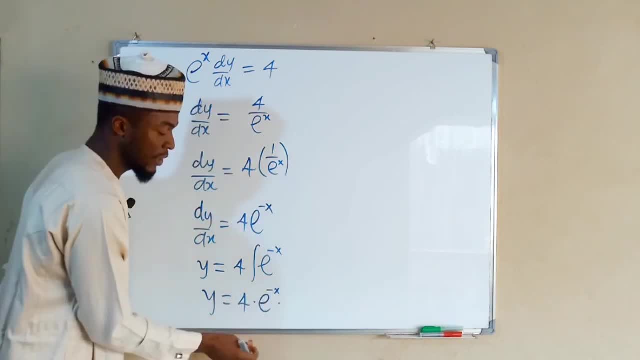 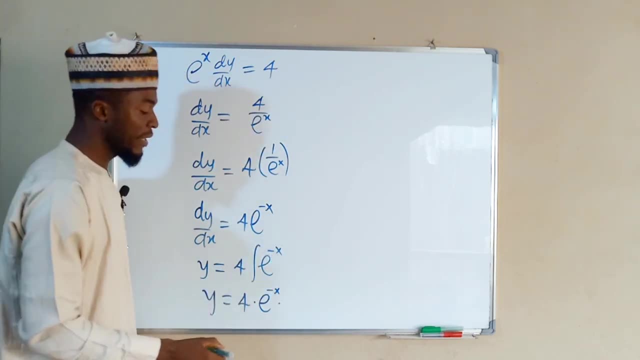 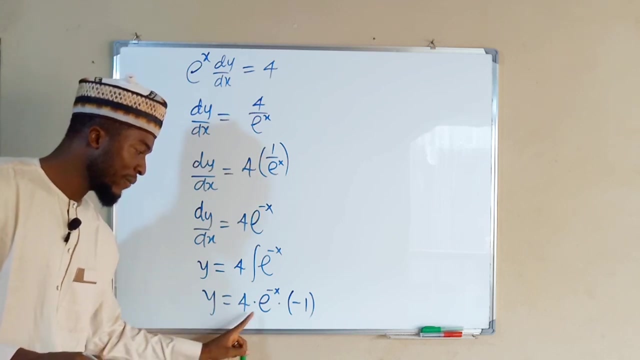 the same thing as the exponential of that function Divide by the derivative of the power of e. If you differentiate negative x, you are going to obtain negative 1.. This is the same thing as multiplying by negative 1 over 1.. So by multiplying them all together, we have negative 4. 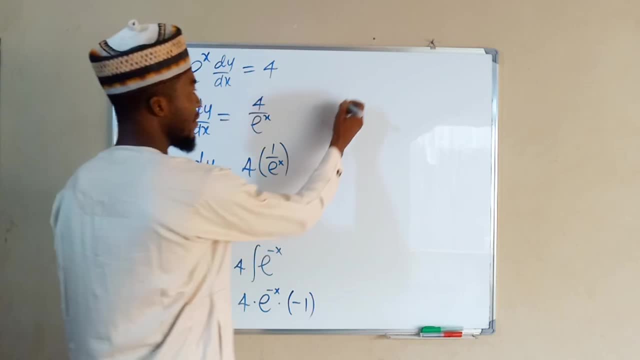 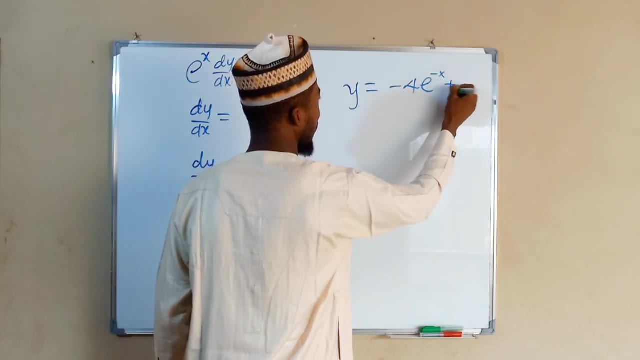 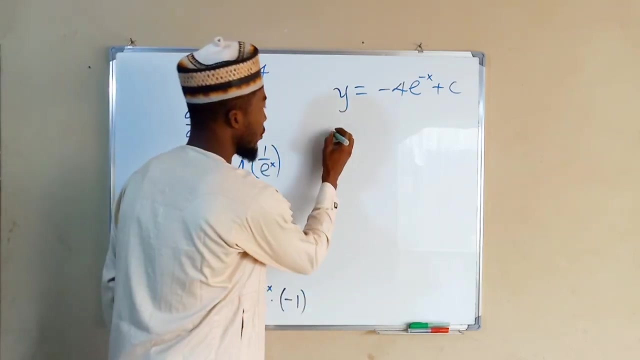 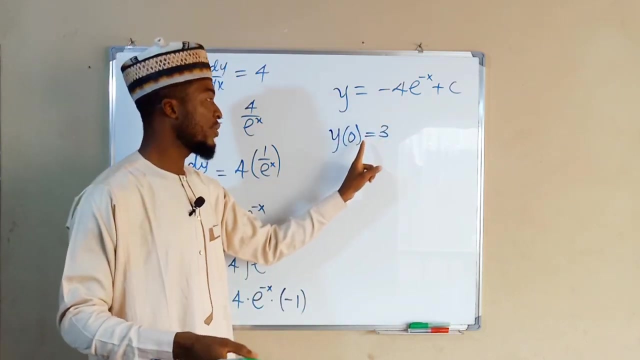 exponential negative x. So therefore we see y equals negative 4 exponential negative x plus the constant of integration c. So this is the general solution for our differential equation. But suppose we are given a condition: y or of 0 equals to 3.. Substituting back in this equation the value of y equals 3 and x. 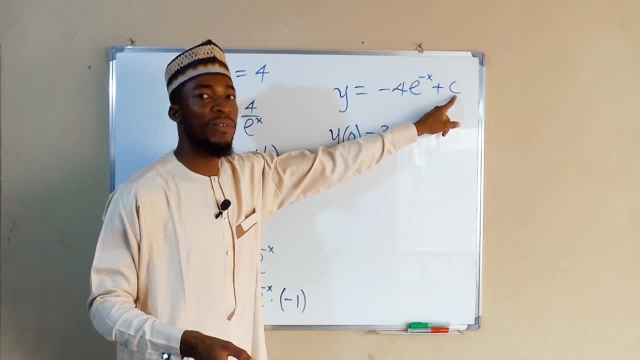 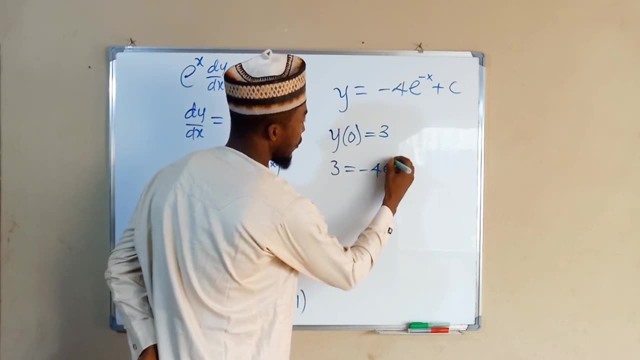 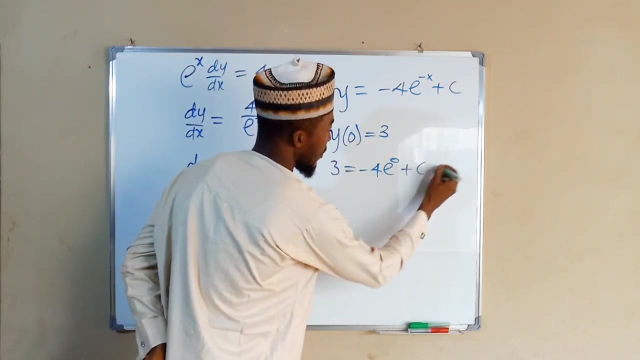 equal to 0. We will be able to find the real value of c. So we see, when y equals to 3, then x equal to 0. So we have negative times. 0 is still 0, then plus c, 3 equals to negative.